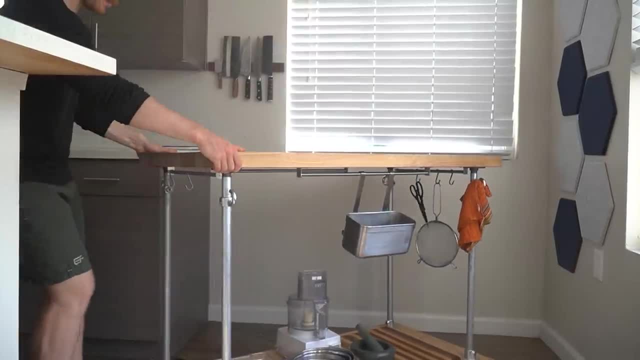 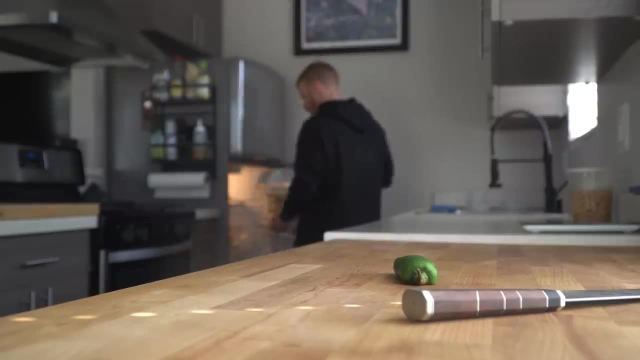 apartment, there was a five foot long area beneath the window, And this is where I've decided to put my movable kitchen island, which was primarily created to be the centerpiece for videos, as well as make more counter space for cooking With my counters, I like to keep them completely clear. 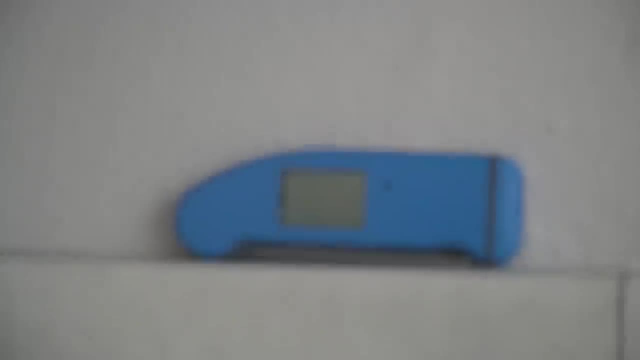 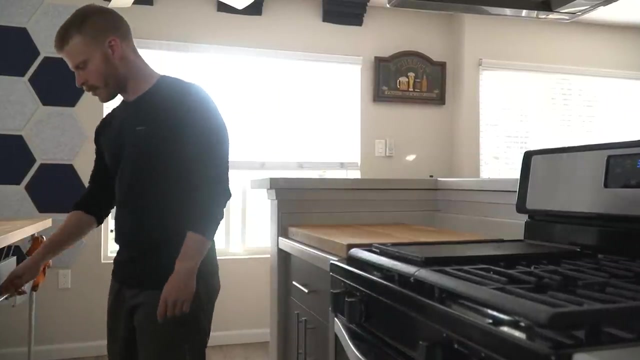 other than small items that I use frequently, which are my thermometer, my scale, my dish drying mat and my salt pig For me, I want to walk into my kitchen and see if there's anything that I need to do in my kitchen and feel like I have this blank canvas to cook upon, because that's when I feel. 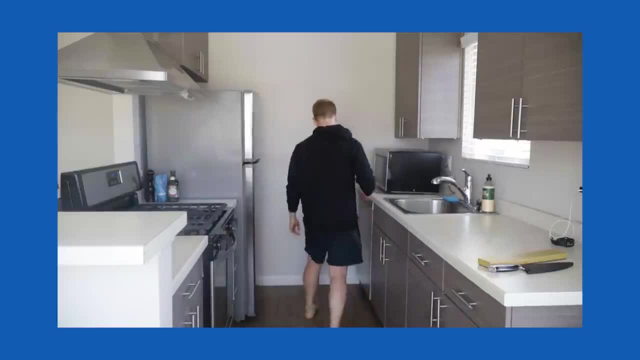 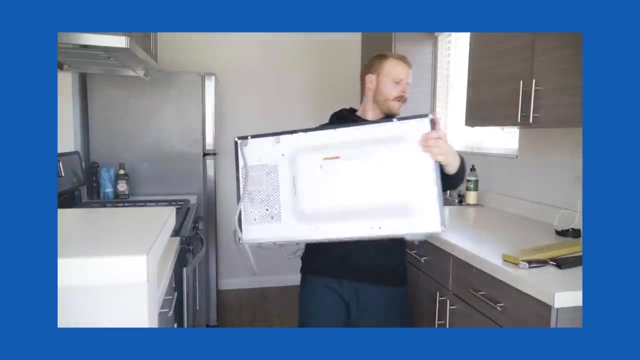 most at ease while cooking. When I moved into this apartment, the microwave was actually taking up the entire counter to the left of the sink. But since I only use a microwave like two to three times a week, it made zero sense for me to actually have it out on the counter all the time, So I moved it. 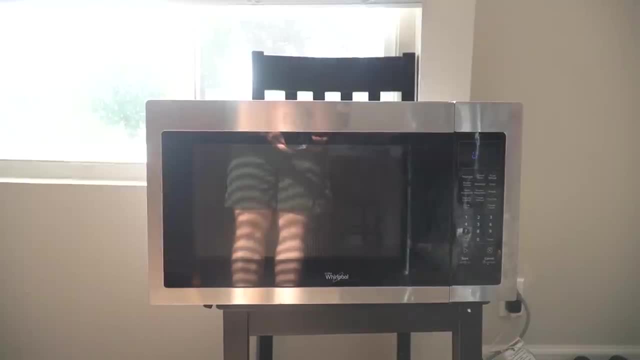 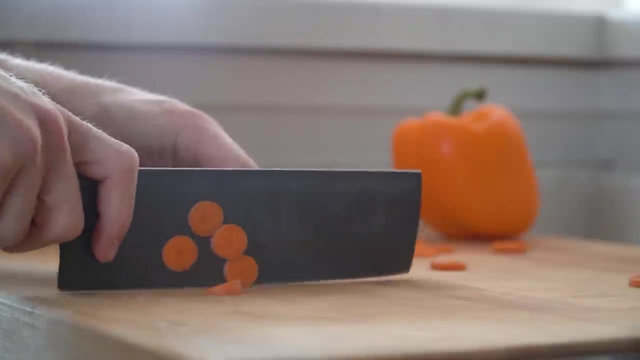 back out to my living room, still deciding on the shelving unit. Lastly, to the left of the stove I set up a large booze block cutting board, and this stays out permanently and is probably where most of my prep work happens for small meals that I'm not filming. This is what I want my kitchen to. 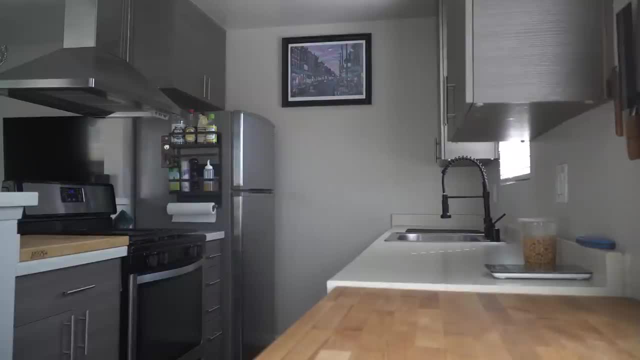 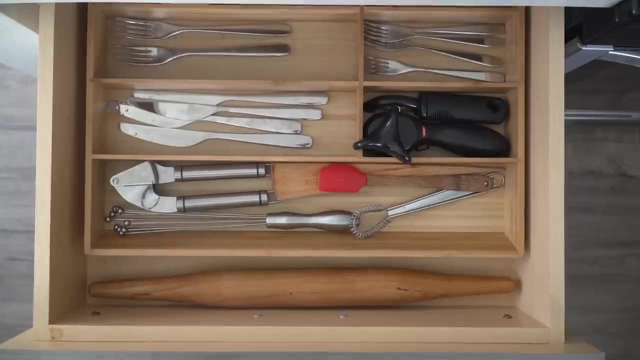 look like after finishing cooking and cleaning. each time Now, with this general layout covered, facing the stove will move left to right around the kitchen. The first drawer to the left of the stove houses my cutlery and some small utensils like a rolling pin, grater whisk, garlic crusher. 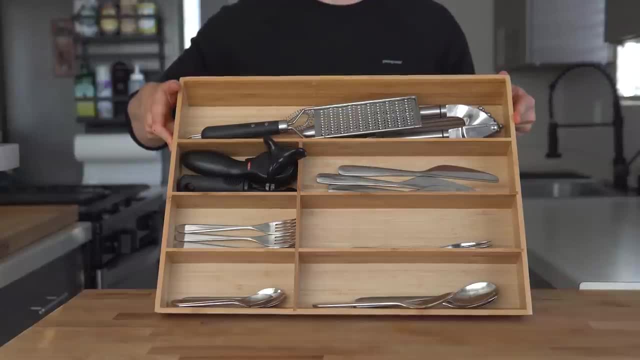 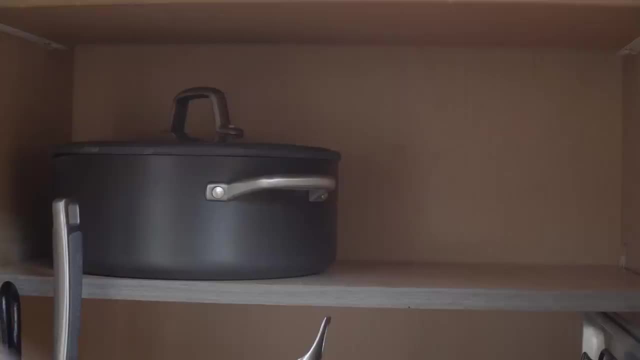 and can opener, And all of these items are just placed in a bamboo drawer. organizer from IKEA. The cabinet below the cutlery drawer is where I store my pots and pans. On the top shelf I have my large stock pot and just a lid to one of. 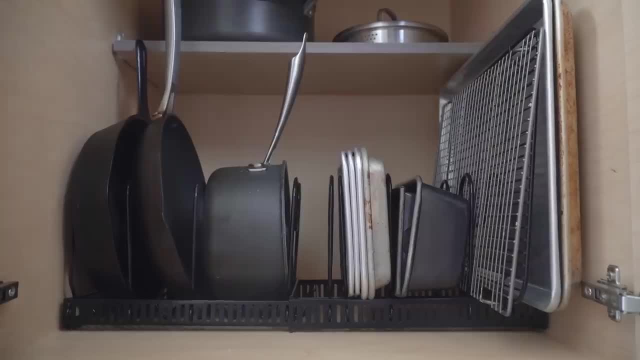 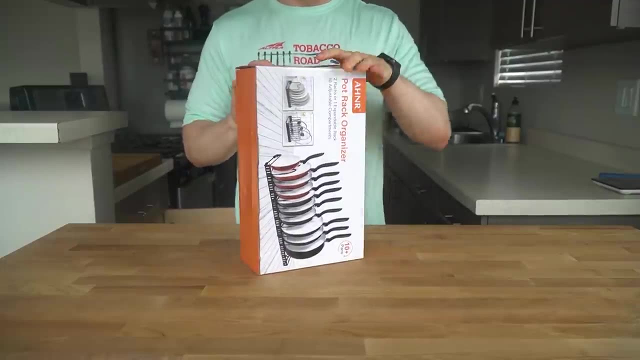 my other saucepans. Then, on the bottom, I have my pots and pans stored in an expandable pot organizer I got from Amazon. It was about $27 and is a game changer for storage. Storing the pans upright instead of stacking them on top of each other makes them easier to see and there's no banging around. 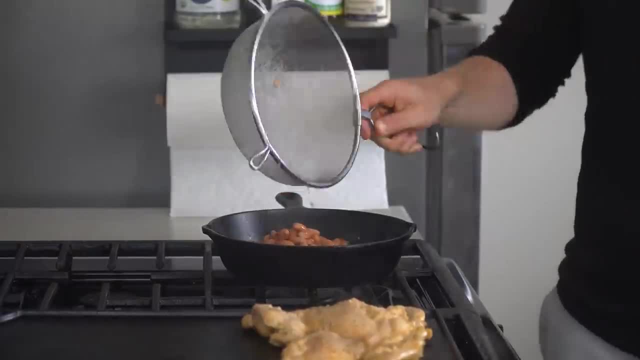 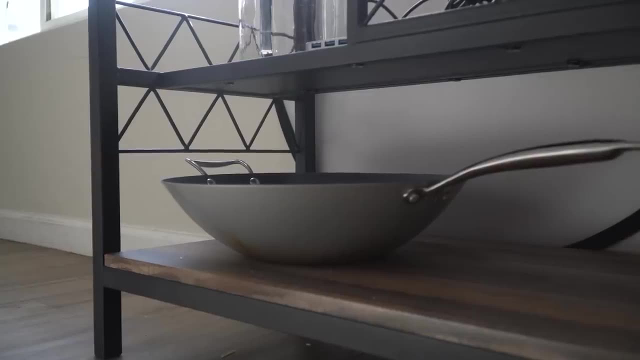 of pots. Another note on my pots and pans. I've tried to keep them to a minimal number, to what I actually need and use. This is all of them, besides my wok, which is too large for this cabinet, and then my cast iron. 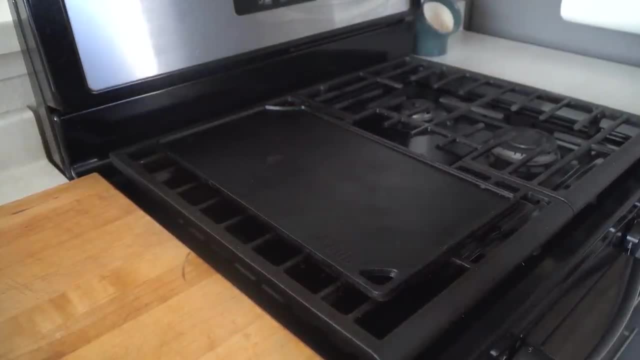 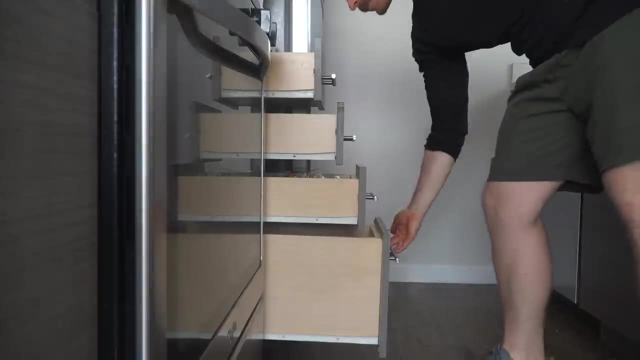 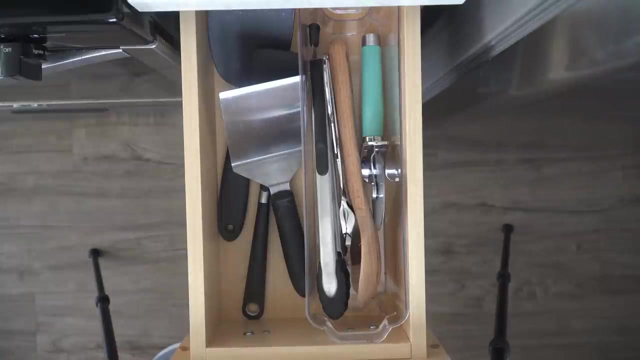 griddle, which I actually can store in here, but it basically lives on top of my stovetop, since it is easily my most used. pan To the right of the stove are a column of four small drawers. On the top it contains my essential cooking utensils, like spatulas, tongs and slotted spoons. Below, 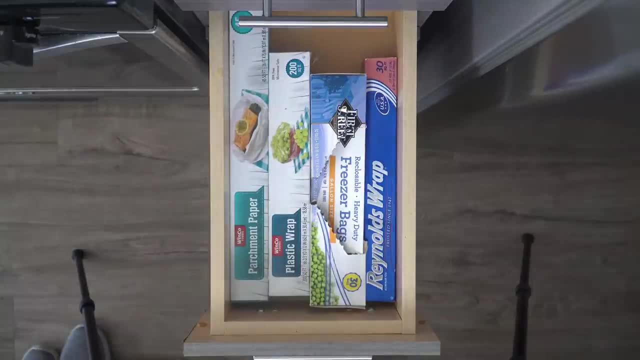 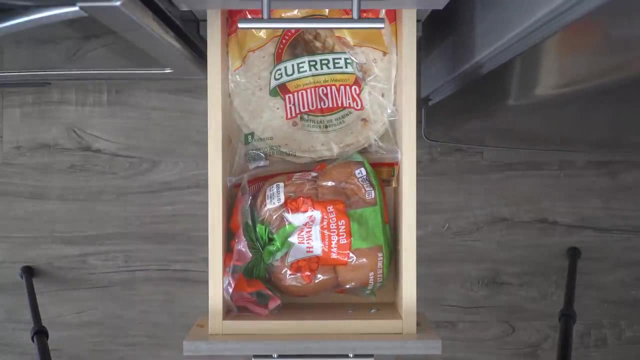 this drawer is my plastic wrap, freezer bags, tin foil and parchment paper. The third one down usually stores breads that are eaten within a couple of days. Right now I just have some flour tortillas and burger buns. The bottom drawer contains all of my deli. 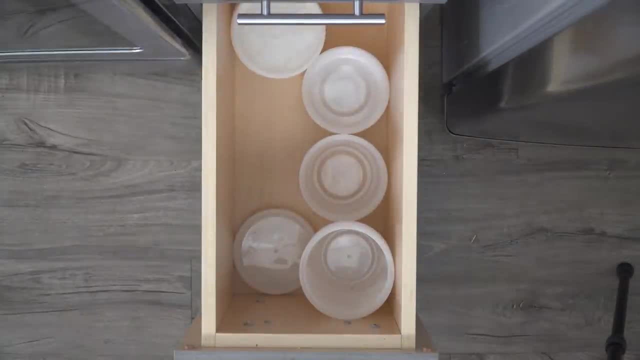 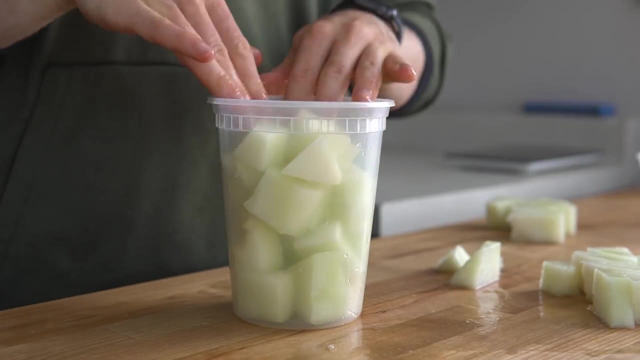 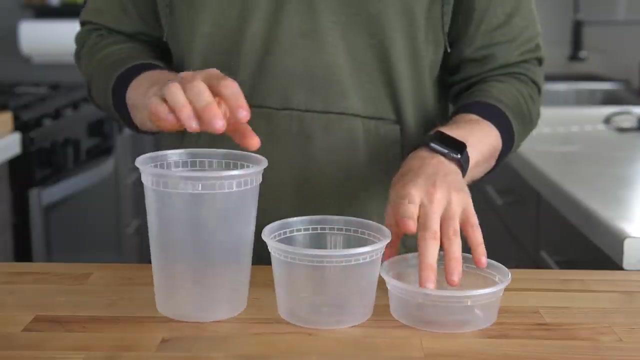 containers, which are the containers I use for basically 95% of storing my food. I switched to these when I moved into this apartment and they are absolutely game-changing. They are washable, reusable. you can recycle them when they have run their course or get stained, and I have them in. 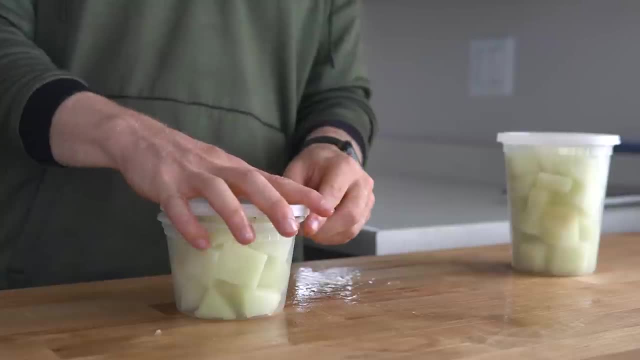 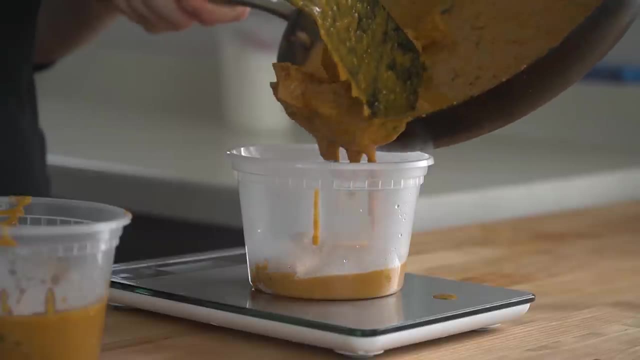 8-ounce, 16-ounce and 32-ounce sizes. I love them because all the lids are the same size and they fit really nice in the fridge. they're easy to see what's inside them, And I do have a couple of glass containers that I'll. 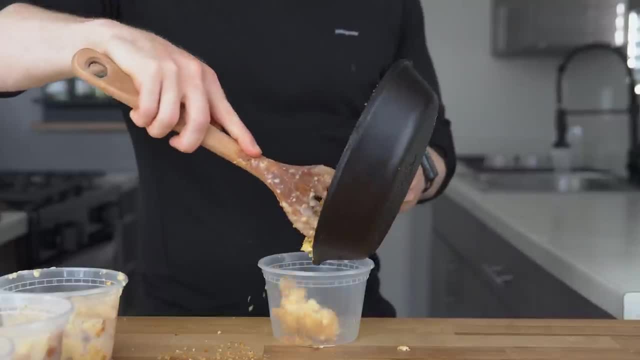 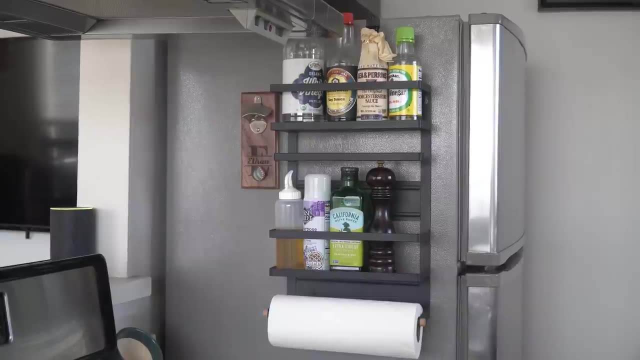 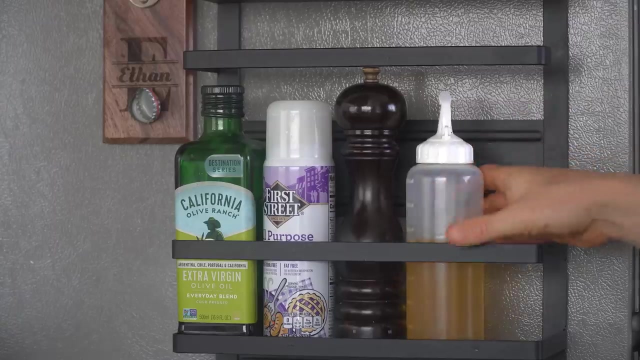 use, sometimes for foods that may fit better in a rectangle, but most of the time I only use these deli container. Now let's talk about the fridge, starting with the exterior. So on the outside of my fridge is a magnetic shelf organizer that I found on Amazon to store my daily use oils. 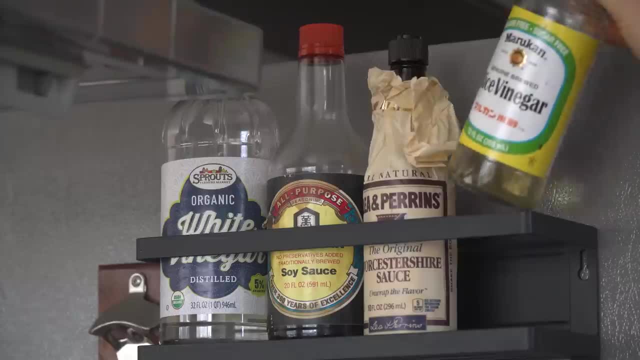 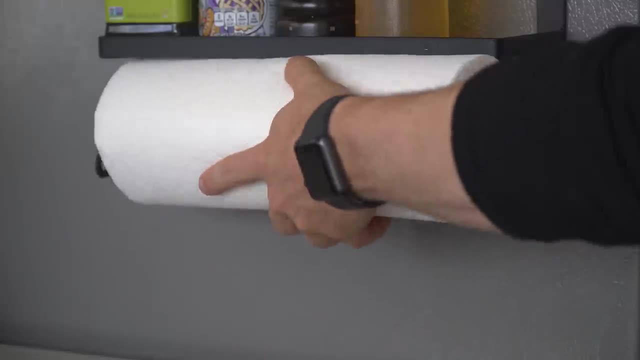 like peanut and olive oil, along with cooking spray and black pepper, And then on the top I keep some sauces and vinegars. It also houses a roll of paper towels and I found it for about $25 at the time, and it's one of my best finds for organization. The magnet is super strong and I 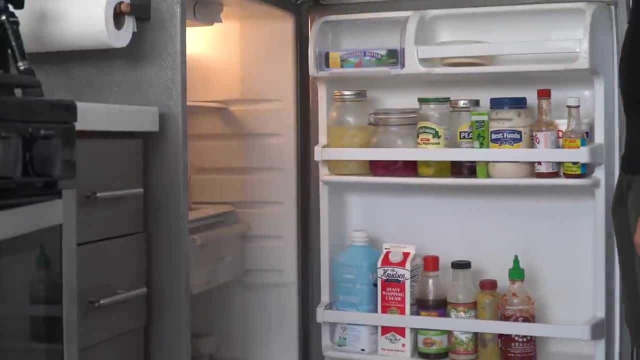 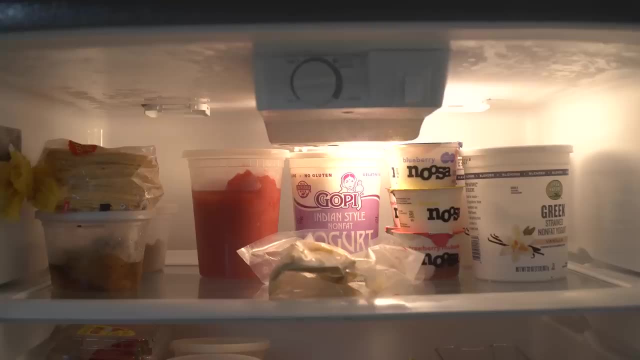 have zero worries about it falling off. but now let's talk about the inside of the fridge. So in general, the top and bottom shelves are the coldest areas of the fridge. So on the top shelf I like to put my leftovers so they can cool faster and get them out of that food danger zone which is 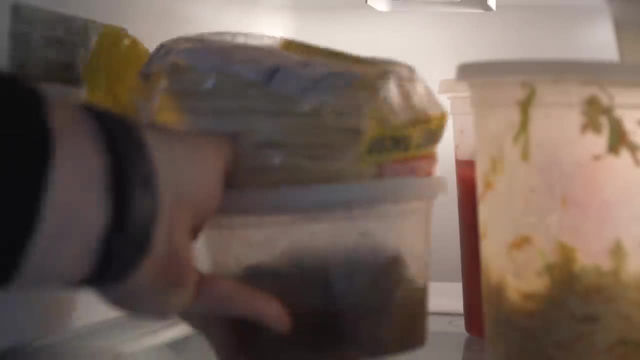 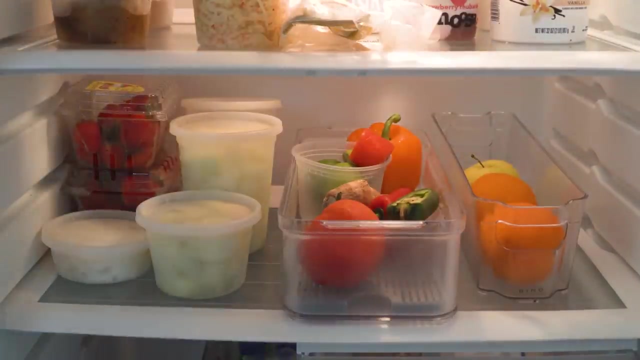 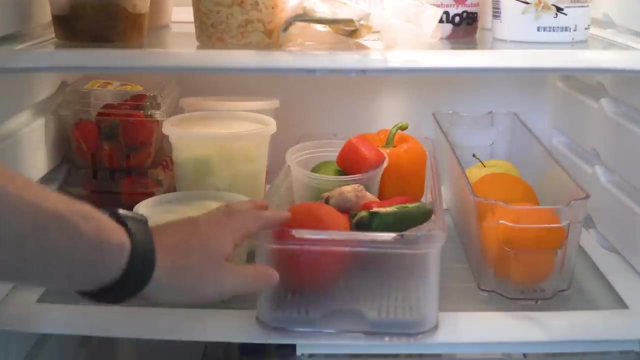 40 to 140 degrees Fahrenheit. I also store my yeast in the back, along with some other things like yogurt On my middle shelf. I like to place my vegetables and fruits in bins. This keeps them semi organized and it's easy to see what I have on hand, Since my eyes are naturally drawn to the 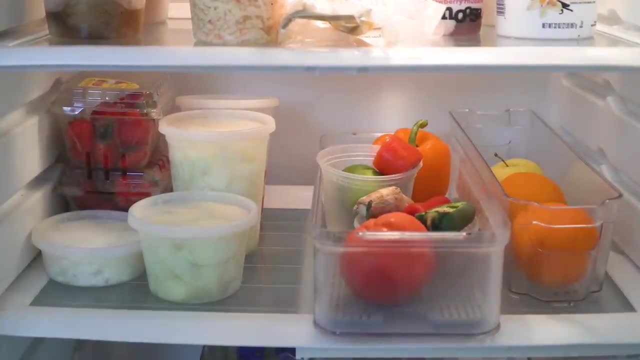 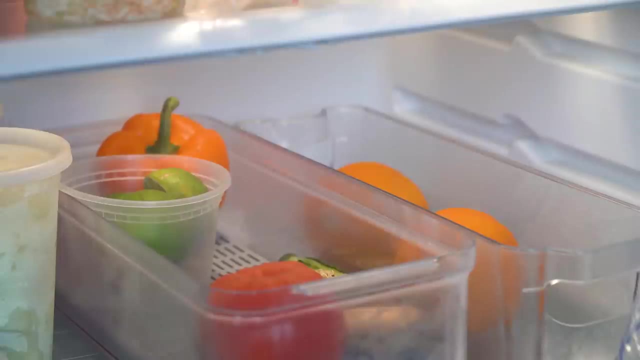 bright colors in the middle of the fridge. I generally find that I use up my fruits and vegetables before they go bad. This is opposed to what I used to do, where I used to just chuck everything in a bin at the bottom and would end up with nothing. So that's a cool thing to know. 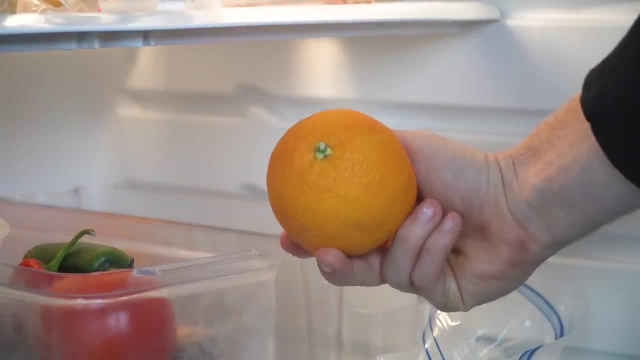 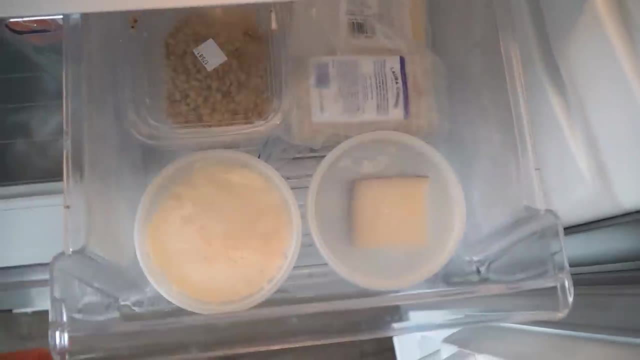 and would end up with a bunch of bad vegetables by the end of the week. On the bottom shelf I like to place items like drinks and my eggs or any overflow items, And then in the shelf drawer I like to keep all my cheeses. 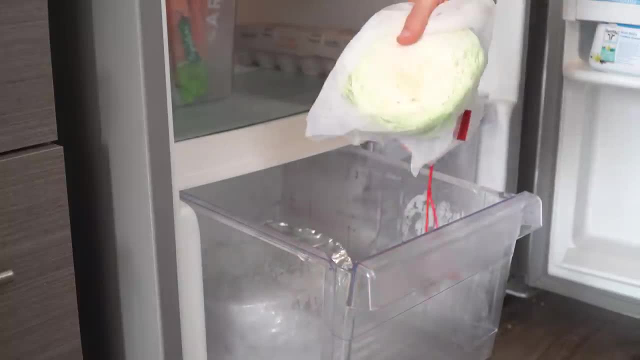 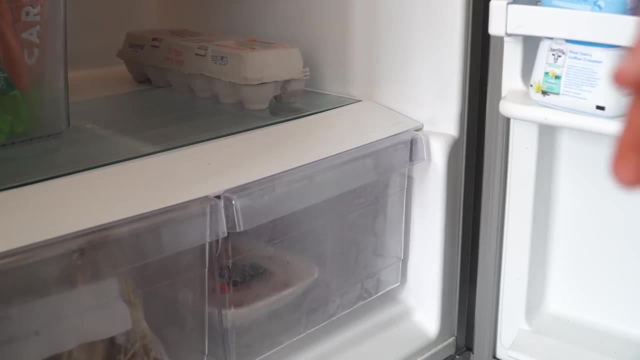 In the large bottom drawers at the bottom of the fridge, I like to place my larger vegetables, like carrots and lettuce, being sure not to overfill the drawer, just so I can make sure I can see everything inside there. And then, lastly, I place all my raw meats. 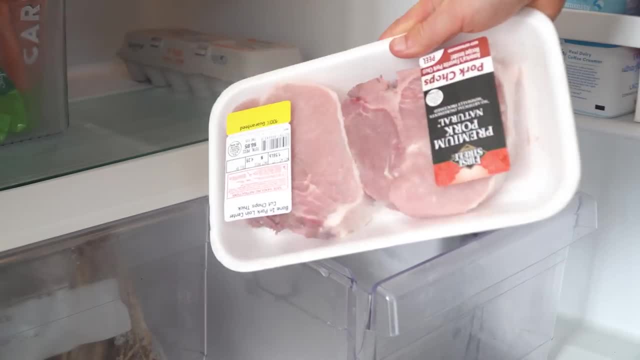 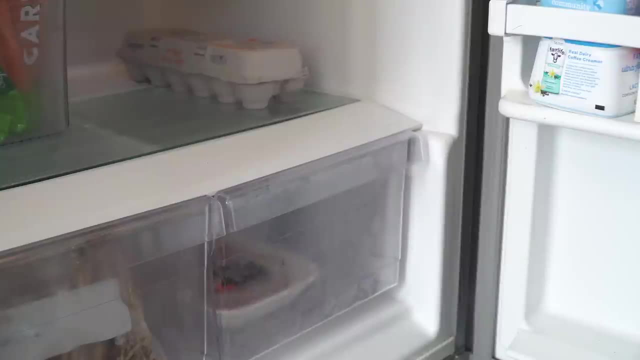 in the lower right drawer. Not only is this my coldest area, but if any drips happen, it's not gonna contaminate any other food in the fridge and it's easily cleaned up in the bin. Lastly, the fridge door is for all of my condiments. 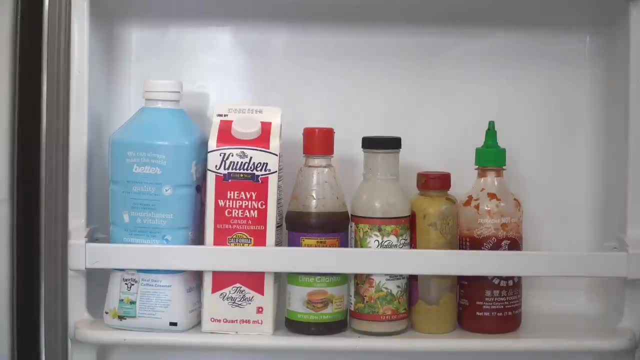 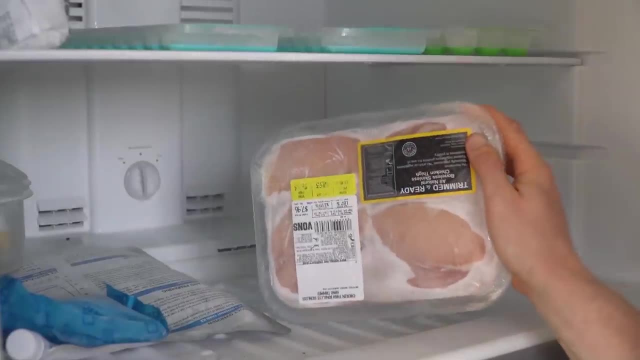 pickled items and drinks. I try to keep them in a single row so none get tucked behind where I can't see them. Then in the freezer I like to keep some pre-portioned leftovers, some meats that I may have got a good deal on. 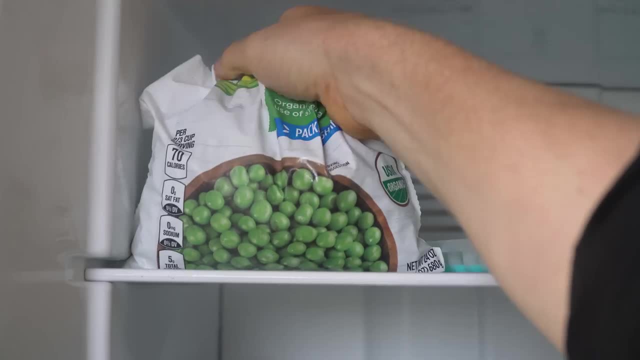 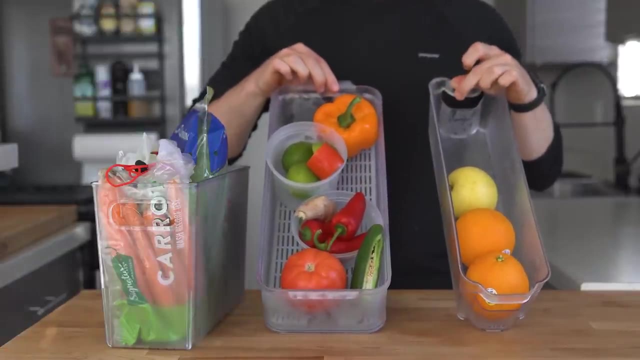 but haven't got a chance to cook yet. ice and usually a bag of peas in case I end up with a black eye. My big tips for the fridge are getting some storage bins like these to provide some separation and organization for your items, instead of just keeping them in plastic bags. 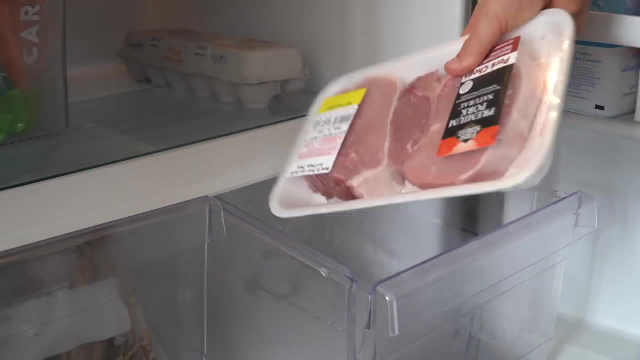 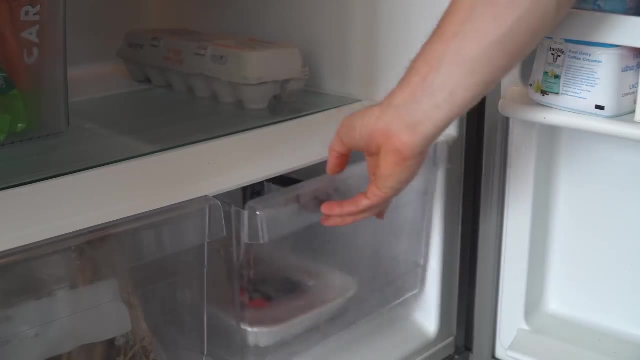 from the grocery store. Also, making sure your raw meats are placed in a drawer, like I do, or at least on a plate, are critical for reducing the risk for cross-contamination. if something were to go bad, Swiveling to the sink side of the kitchen. 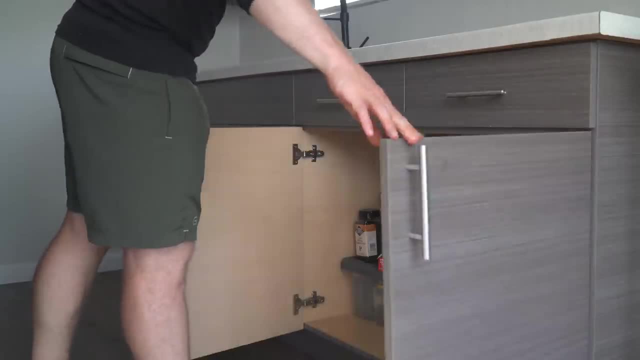 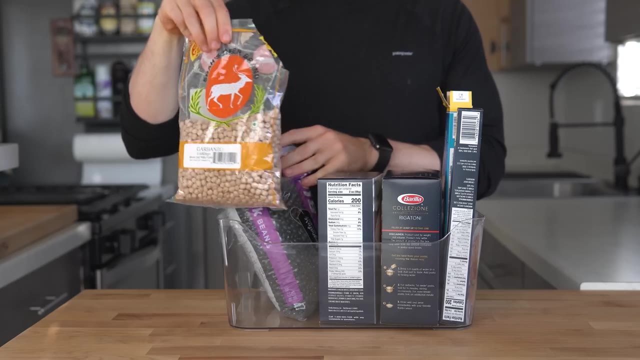 we have the pantry, which is part in this cabinet and part of the lower cabinets to the right of the sink. Now I used to stock up on a ton of stuff, but I've since kind of abandoned that approach so I can get better at actually using what I have. 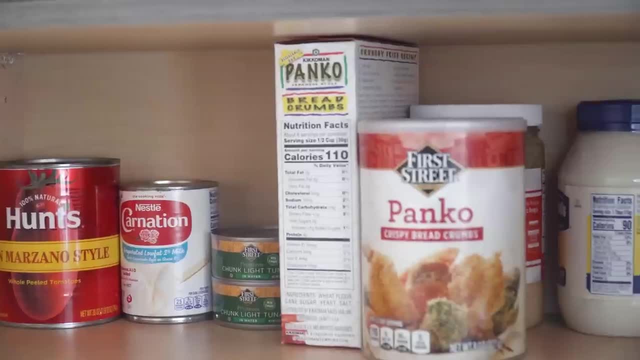 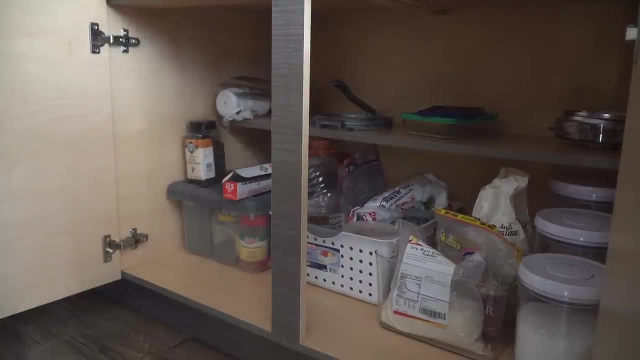 Typically you'll see things like whole tomatoes, evaporated milk, plenty of pastas and various vinegars and other sauces. Then in my pantry cabinets to the right of the sink, I have my leftover spices that I use to refill my spice bottles. 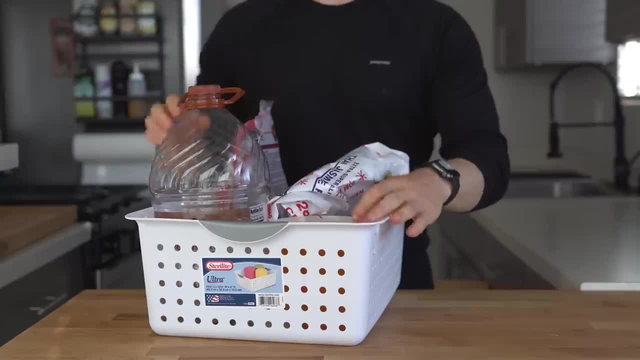 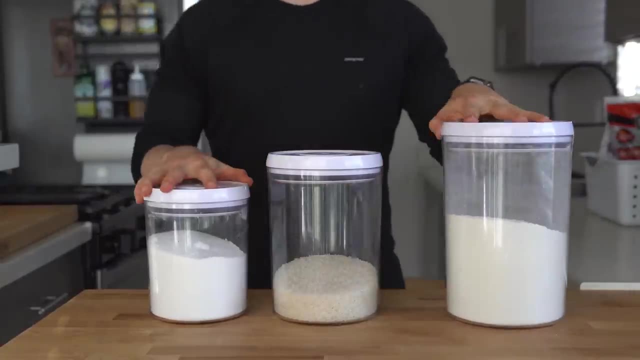 spices, like dried chilies, that I may not use very often, and then I also like to keep my excess peanut oil, baking items like cornmeal, cornstarch. and then I have these resealable containers from OXO that have my bread, flour, sugar and rice. 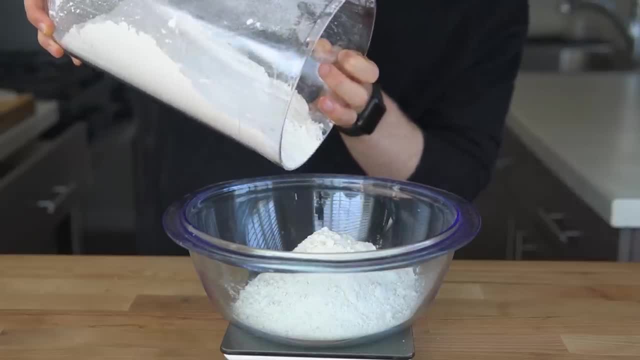 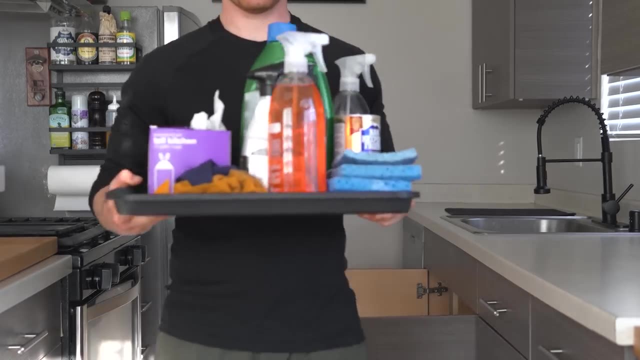 These are really nice containers for pantry items that I would highly suggest For the sink. I did a video about the install if you want to check it out. but for organization-wise, I just have this dish mat out that has my sponges- dish soap. 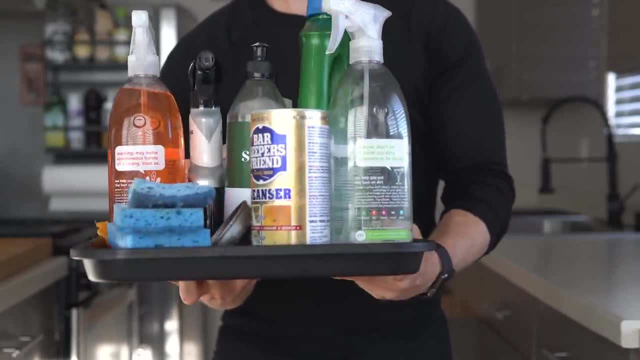 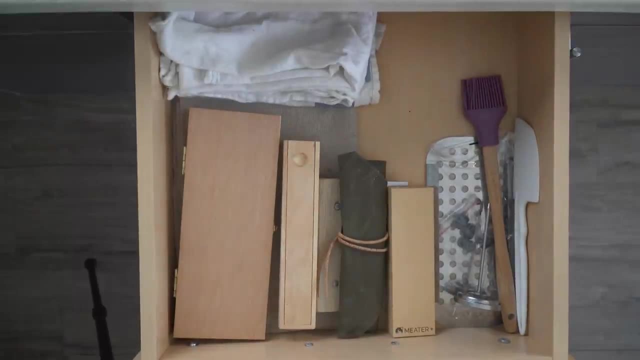 trash bags, barkeeper's friends and some general purpose spray under here, and then I also keep my trash bin under the sink as well. To the drawer to the right of the sink, I just have some various items, like some extra towels. 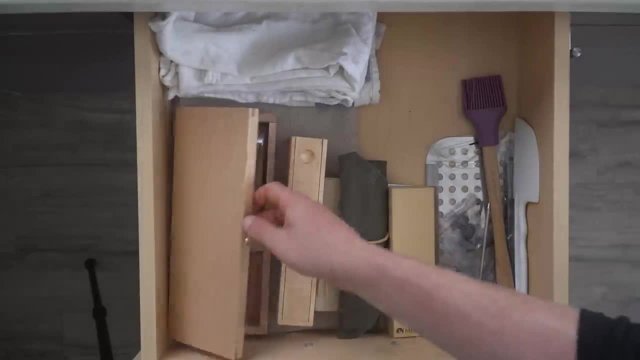 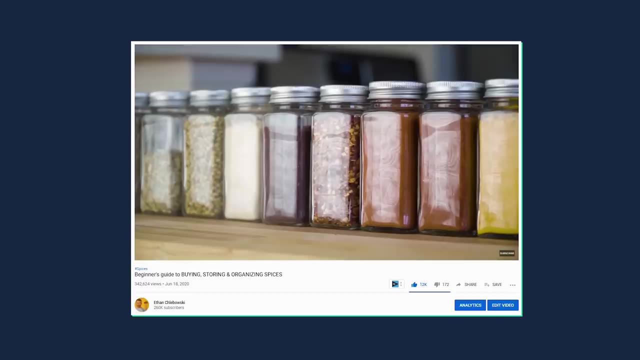 some bread-making items and like an extra thermometer or something, but to the drawer to the right of that one I have all of my spices, So I did a whole video if you do want some more in-depth information about what spices I use. 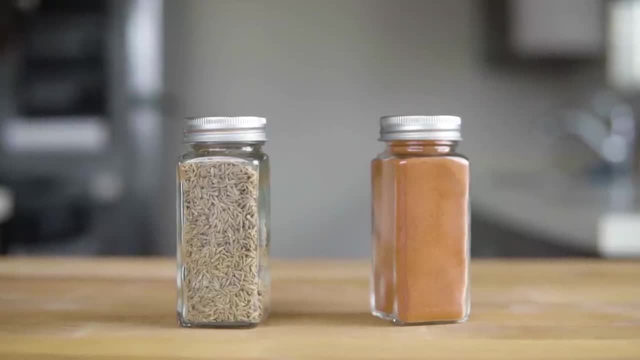 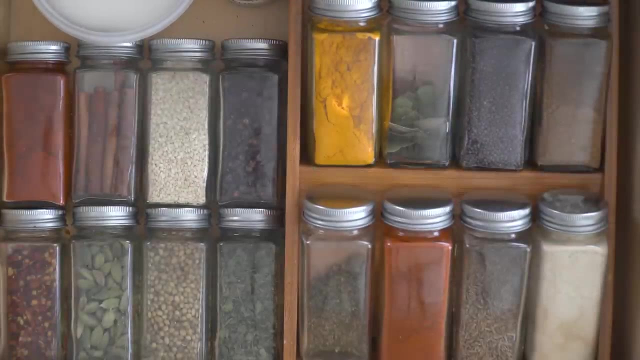 but in general you just want to keep your spices away from open air, moisture, heat and direct light. So I decided to keep mine in translucent jars, just because they look cool, but store them in this drawer. They are easily refillable. 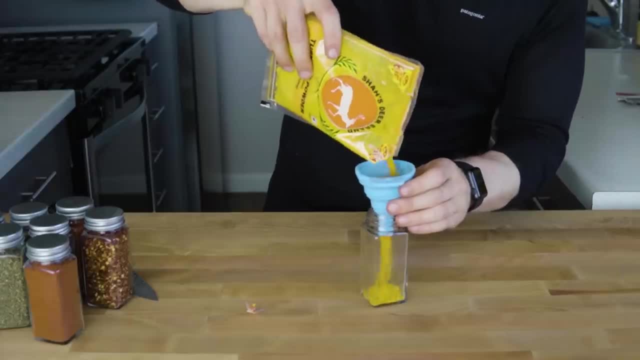 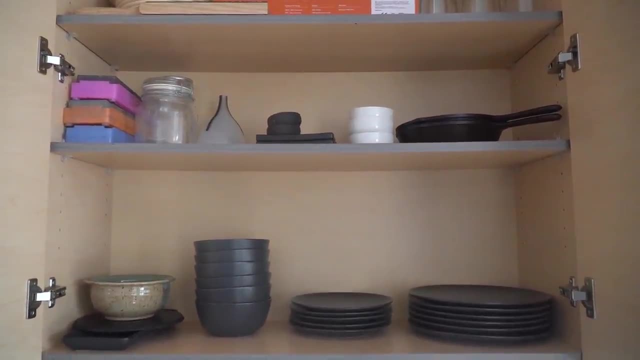 and easily identifiable For my table and dishware. I keep it in this large cabinet and plates and bowls are on the bottom shelf, which I use most often. Then on the second shelf I have my whetstone, some other plates, 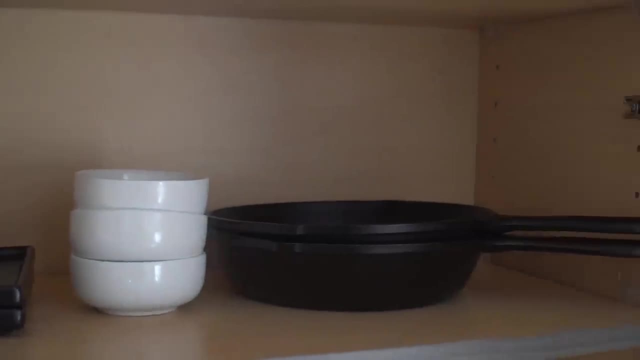 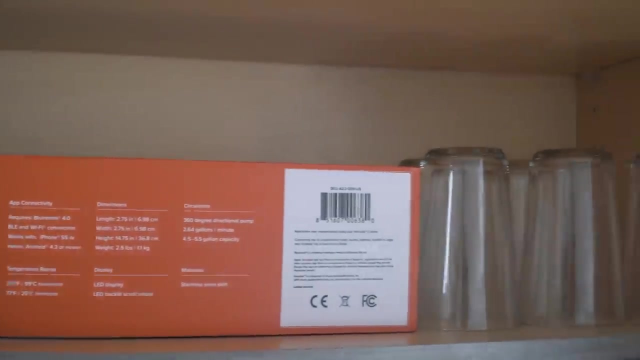 mason jars for pickled onions and some cast irons for plating purposes, like in my mac and cheese video. Then on the next top shelf I have some bread baskets, a sous vide and some glasses. Nothing on the top shelf. 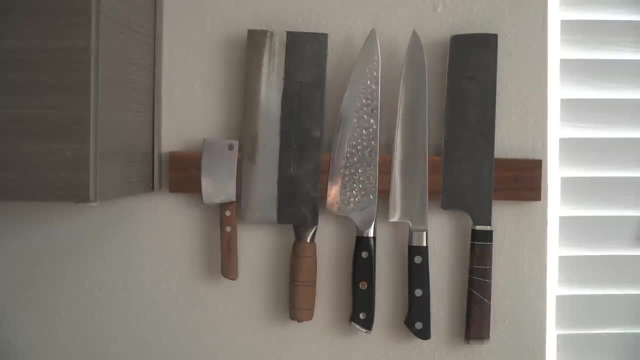 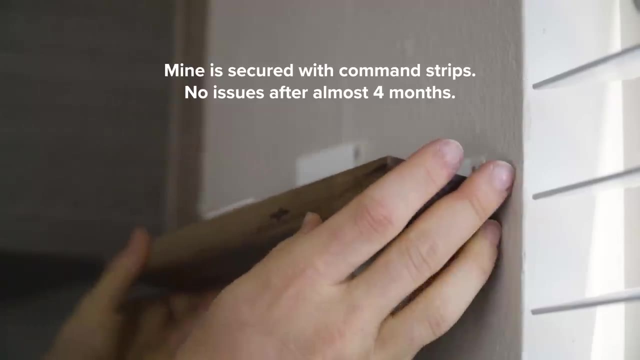 because I can't reach it To the right of the cabinets for knife storage, I went for a magnetic wall rack. Now, this is not only a sexy way to show off your knives, but it's also probably the best storage technique because it won't dull the edge. 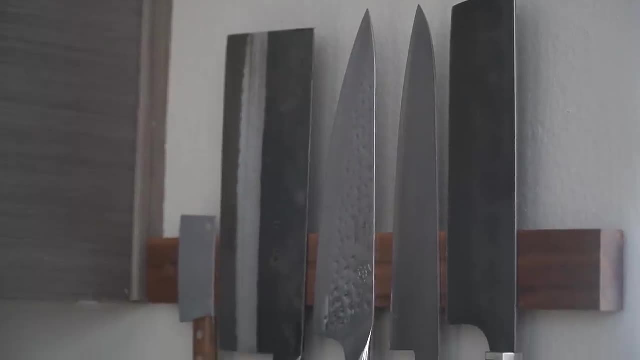 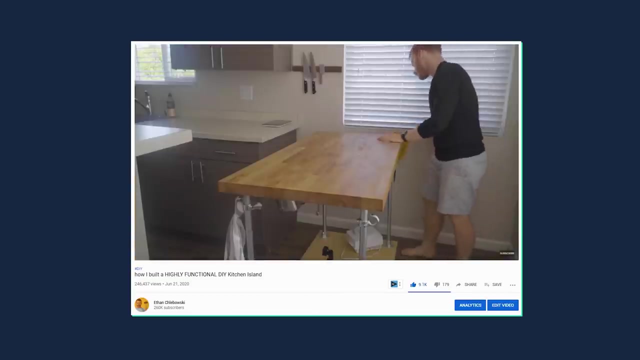 like a knife block might, and if some water is left on the knife, it will dry out instead of mold or mildew potentially developing. To round out, the tour is again my DIY kitchen island. Again, it's just the centerpiece for my videos. 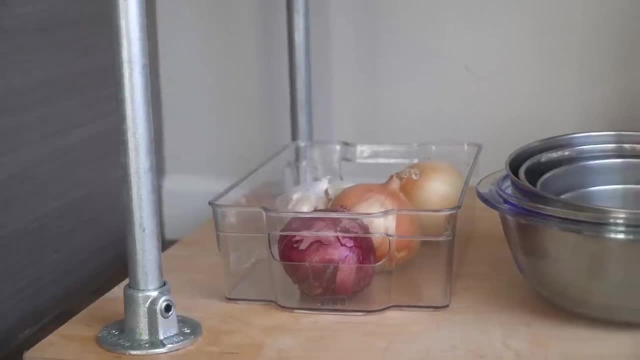 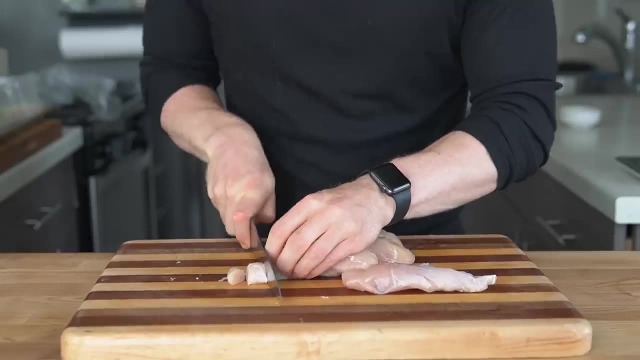 but I do store a couple of things underneath here, like my onion and garlic bin, which I use all the time, some mixing bowls, my food processor, my mortar and pestle and an extra cutting board that I typically use for raw meats. 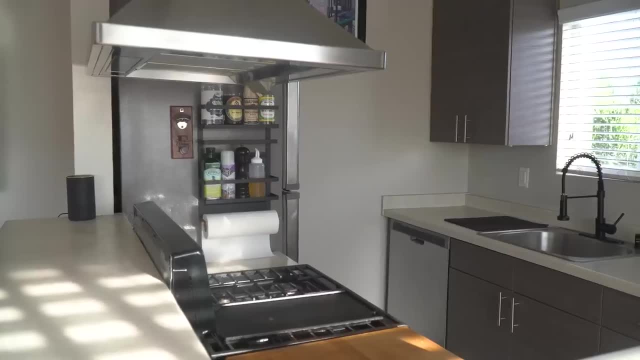 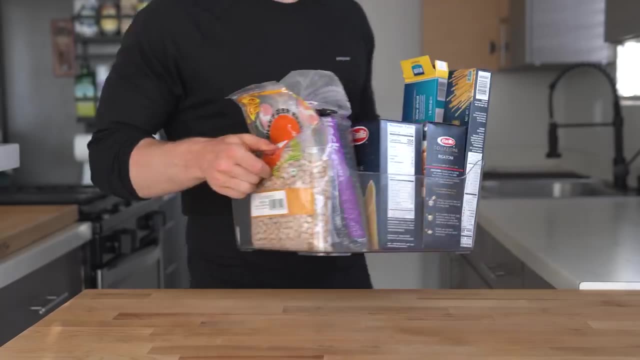 I also do hang a couple of things up here as I see fit, but all in all I've really been liking this system that I put in place for storage and organization in my kitchen. Hopefully you all have found at least one or two things.